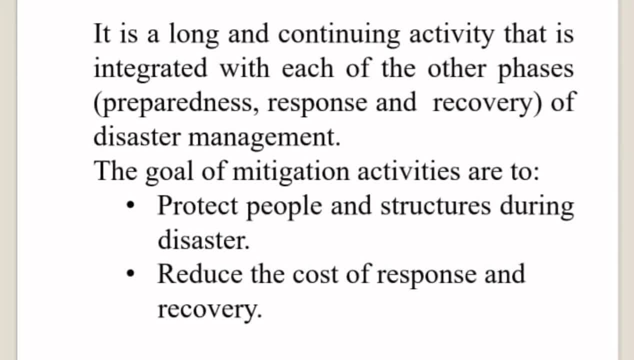 Mitigation is a long and continuous process Which helps us in all the other stages of disaster management, like Preparedness, Response and Recovery. Which helps us in all the other stages of disaster management, like Preparedness, Response and Recovery. And if we talk about the goal of Mitigation Activities, 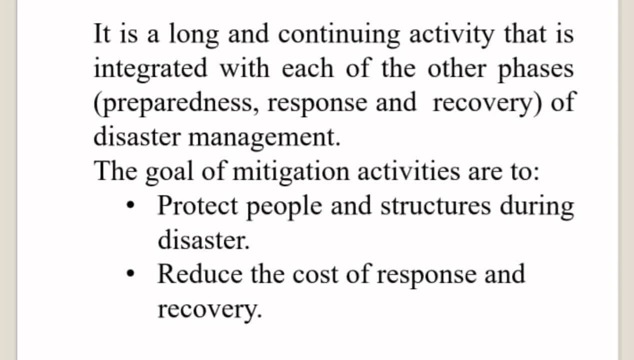 Then the main objective of Mitigation Activities is to protect people and structures during disaster, Meaning to protect human life and property during any disaster. And second goal is to reduce the cost of response and recovery. Meaning to reduce the cost of response and recovery. 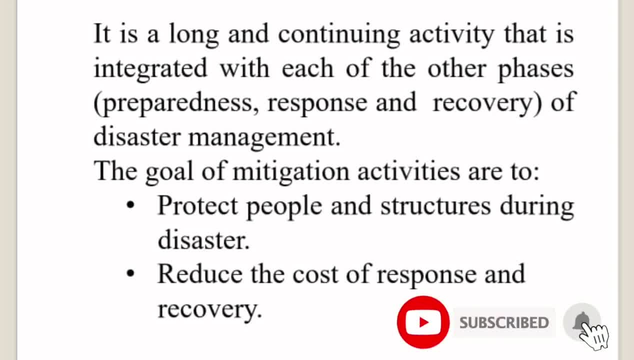 Meaning to reduce the cost of response and recovery, Because the better we follow Mitigation Activities, the less loss we will incur from any disaster, Whether it is loss of human life or loss of property, And because of the less loss, the cost of response and recovery during any disaster and after the disaster will be reduced. 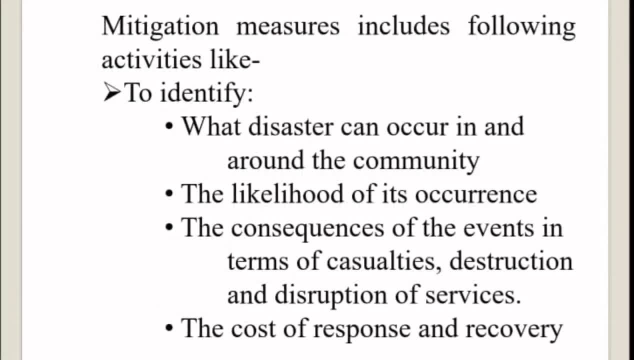 And because of the less loss, the cost of response and recovery. And because of the less loss, the cost of response and recovery. And because of the less loss, the cost of response and recovery. So some Mitigation Activities are used to protect from any disaster. 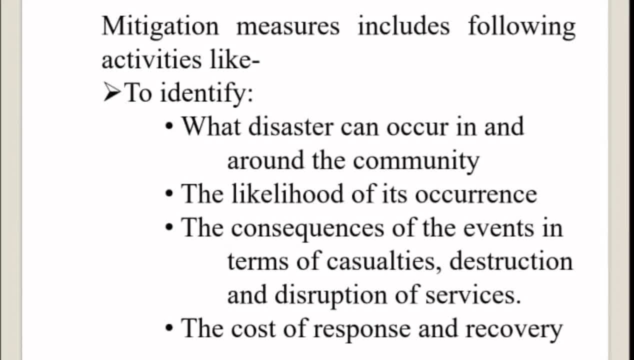 Or to reduce the cost of response and recovery. Third, the consequences of events in terms of casualties, destruction and disruption of services. It means knowing how much loss a community will incur due to a disaster, whether it is a loss of human life or a loss of property. 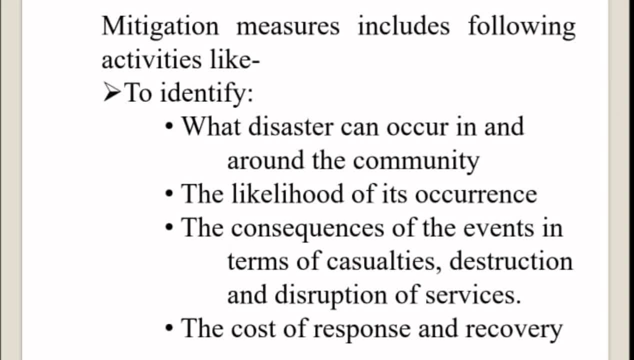 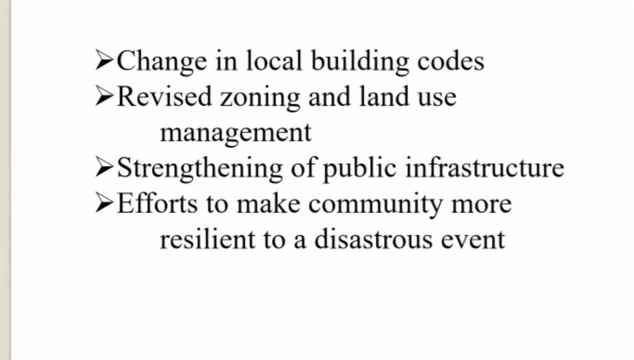 Apart from this, cost of response and recovery, ie the response to a disaster and the improvement that is to be made in the future, is estimated. other than this change in local building codes, ie in some areas the rules of building construction should be changed in this way: 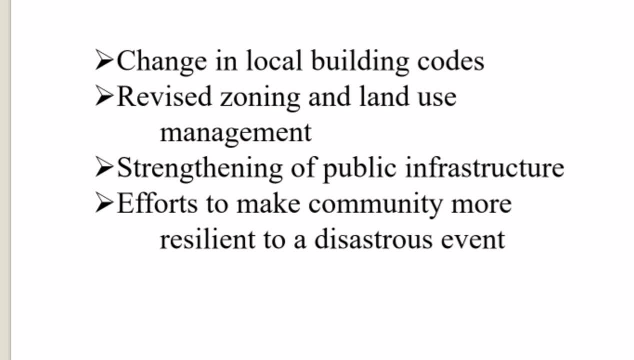 so that at least a loss of human life and property is incurred during a disaster. For example, suppose there is an area where the probability of an earthquake is very high or there are frequent earthquakes. then the construction of a new building is made there like this, so that at least a loss is incurred during a disaster or because of an earthquake. 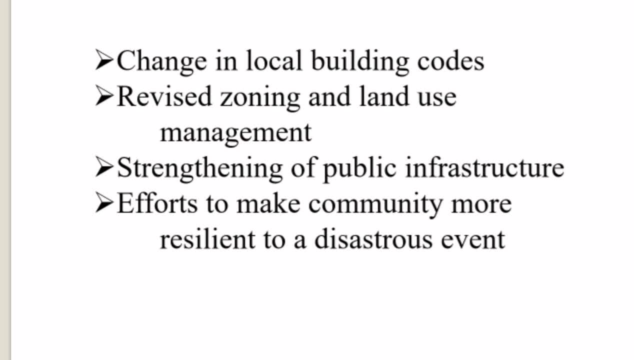 And if there is an area where the probability of an earthquake is high or a loss of property is incurred during an earthquake, then the construction of the buildings that are built there will be done in this way so that the loss of human life and property is reduced. 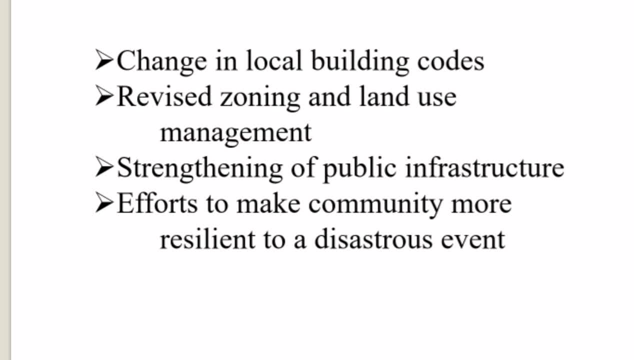 due to a disaster like an earthquake. Revised zoning and land use management, in which the proper management of land and land use is included, so that the damage caused by any disaster can be reduced. Apart from these, public infrastructure such as bridges, roads and public buildings should be strengthened, and the community should be prepared for any future disaster under mitigation measures. 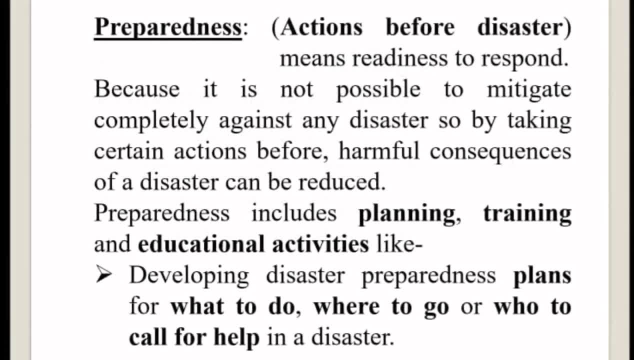 Next is Preparedness, which is a process before a disaster, in which a community is prepared to respond during a disaster, because it is not possible to completely mitigate a disaster. Therefore, in order to reduce the damage caused by a disaster, some preparations have to be made before a disaster, in which planning, training and management are required. 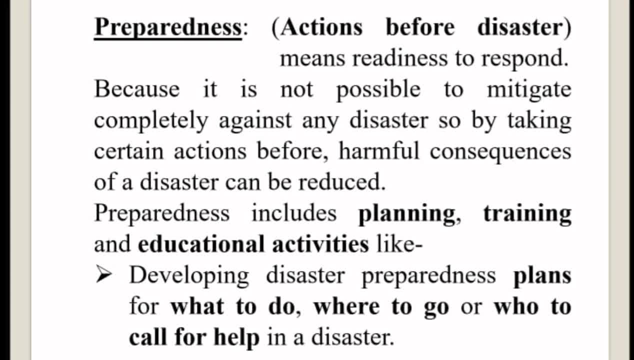 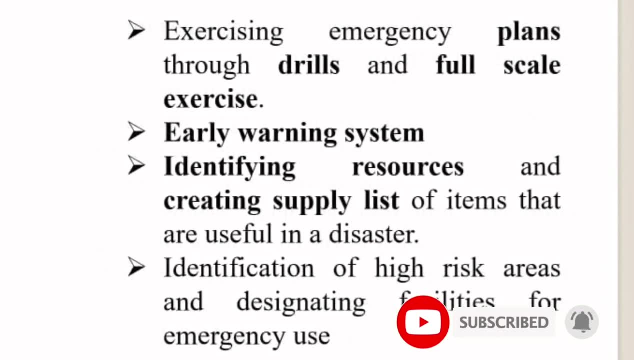 In addition, educational activities can be included, such as making a disaster preparedness plan so that, during a disaster, we can decide what to do, where to go and whom to call for help. Next, the disaster preparedness plan and emergency plan should be practiced periodically through drills or full-scale exercises. 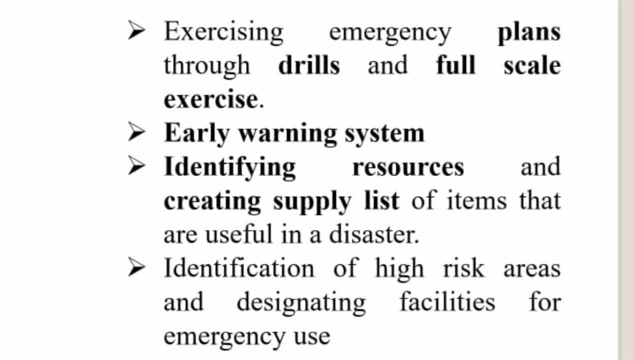 Next, the disaster preparedness plan and emergency plan should be practiced periodically through drills or full-scale exercises. Next, the disaster preparedness plan and emergency plan should be requires brief introduction to resources, including recognising resources and making an актив list of necessary materials for insgesamt use during a disaster. 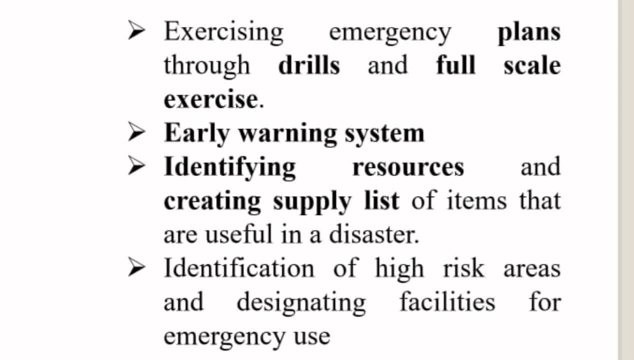 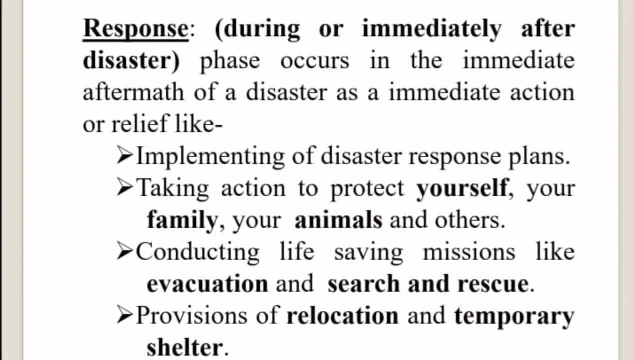 Visitors should be identified with the high risk areas and interacting with emergency facilities in order to discuss solutions with the community. Next, the third stage of disaster management activities is response, in which actions will be taken, one after the other, or or during an emergency, to stop the disaster. 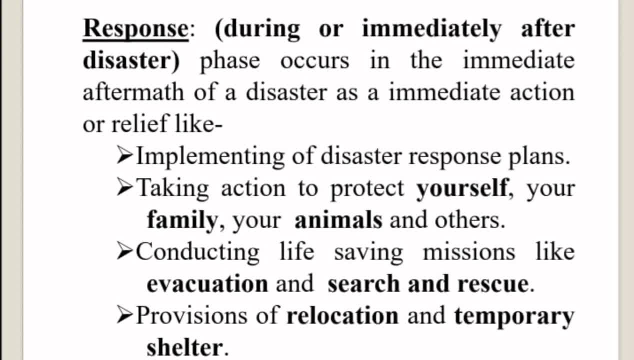 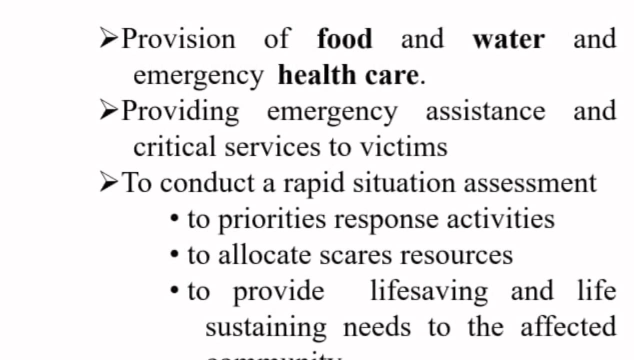 Disaster Response Plan: Implementing Protecting your family and animals, Relief and rescue work, Leaving the affected area and going to a safe place and arranging a temporary shelter there, Providing food, water and emergency health care facilities to people affected by the disaster, And to evaluate the situation of the disaster as soon as possible. 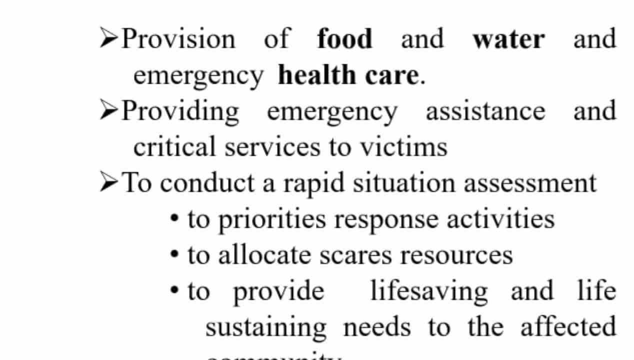 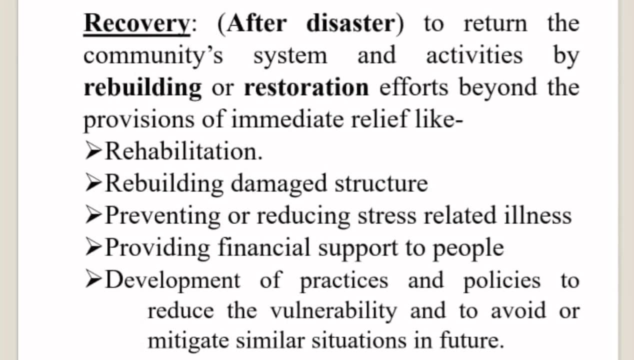 So that the response activities carried out during the disaster can be given priority, The resources available there can be distributed properly And the needs of the community affected by the disaster can be met. Last is recovery phase, In which the reconstruction and repair work carried out after the disaster is included. 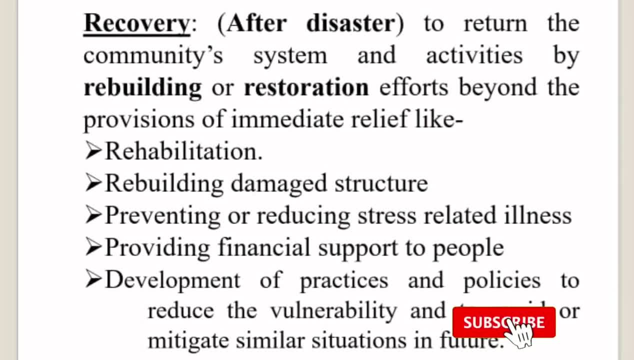 Through which social arrangements or social activities Can be done. normally, as before, It includes the provisions like Rehabilitation, Reconstruction of broken buildings due to the disaster, Giving financial aid to people affected by the disaster So that their mental and financial situation can be improved. Apart from these, such practices and policies are made. 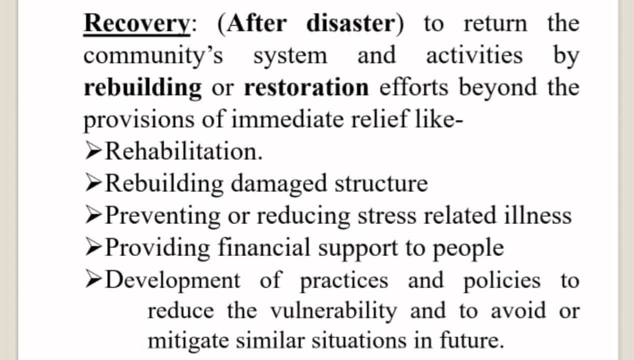 Through which the community's insecurity against any disaster Can be reduced And in the future such a future disaster can be prevented. So we can say that the disaster management is a specific area in itself Under which the human life and property loss from the disaster Or from the methods to be done to reduce. 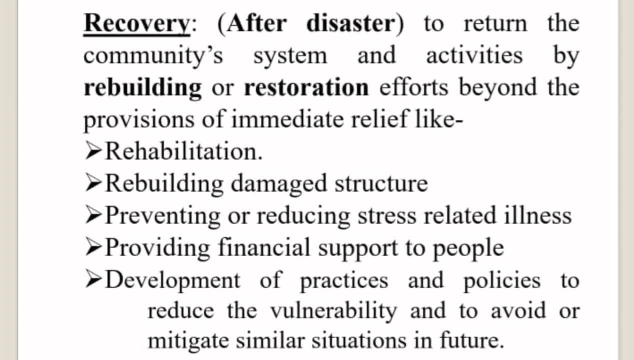 Preparations made prior to the disaster And the measures taken during the disaster And the improvement after the disaster are included.